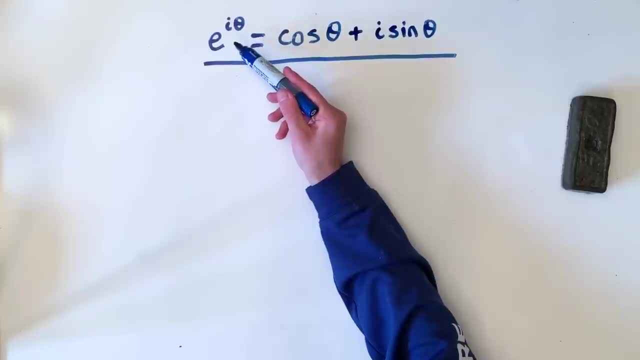 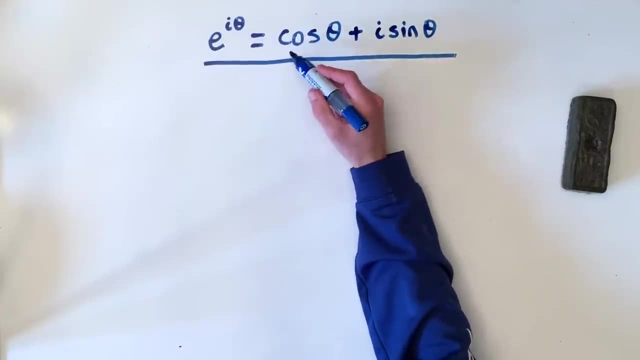 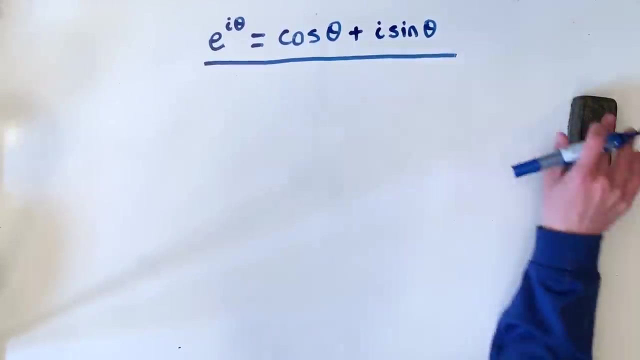 of proofs of people expanding e to the x using a Taylor series approximation and then rearranging the infinite sum to prove that is equal to the cosine of theta plus i times the sine of theta. So instead of doing that, I'm going to set the cosine of theta plus i times the sine of theta. 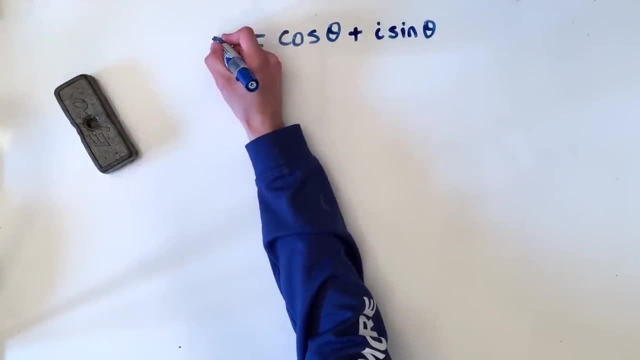 equal to some complex function, z. So we're going to let z equal cosine of theta plus i times the sine of theta. Then I'm going to solve for dz over d theta, or the first derivative of z, and that's going to be equal to. 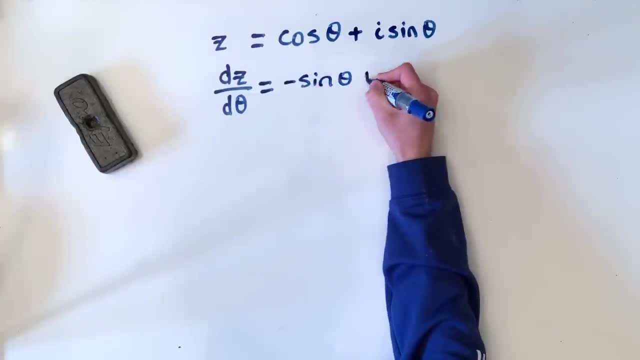 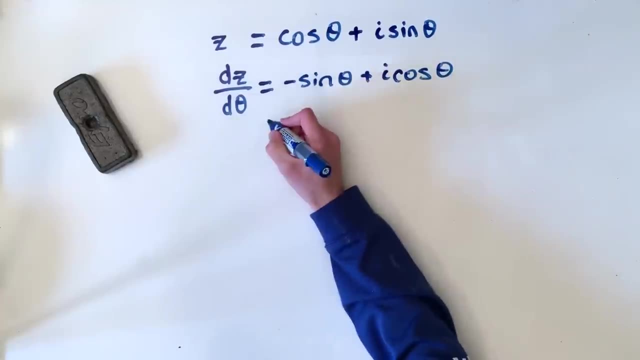 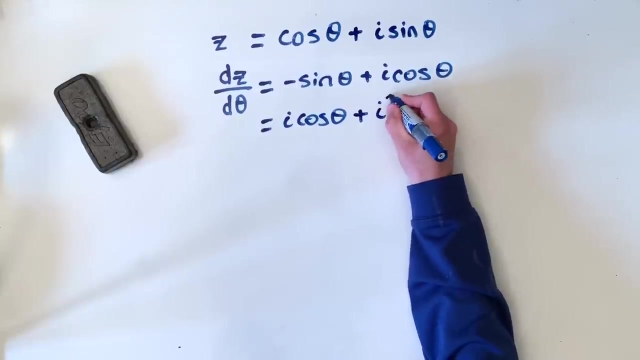 the net derivative of z. So I'm going to write z to the negative sine of theta, plus i times the cosine of theta. And if we rearrange that where we put i times the cosine of theta and instead of writing minus sine times theta, I'm going to write that negative 1 as i squared, as i squared is equal to negative 1.. 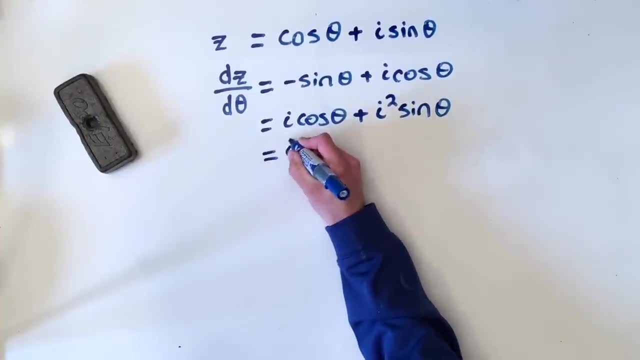 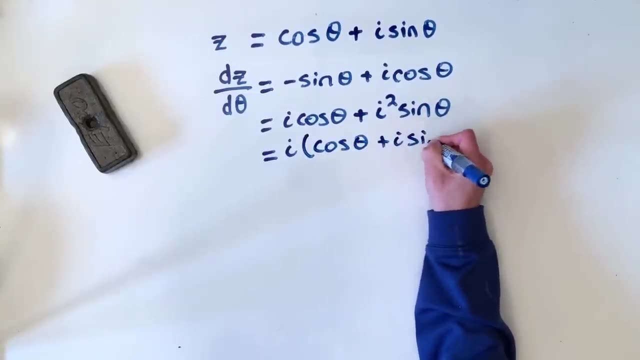 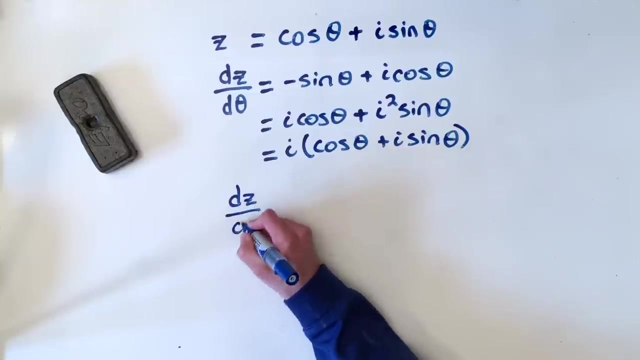 Like that. And then I'll factor out the i from both terms and we'll have cosine of theta plus i times the sine of theta, Like that. And now this is actually our zed right here. So I have just proved that dz over d theta is equal to i times zed. 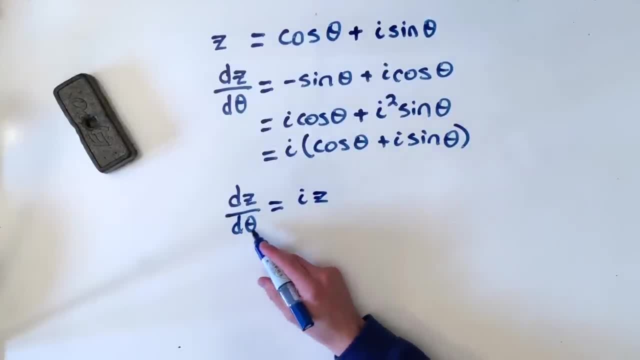 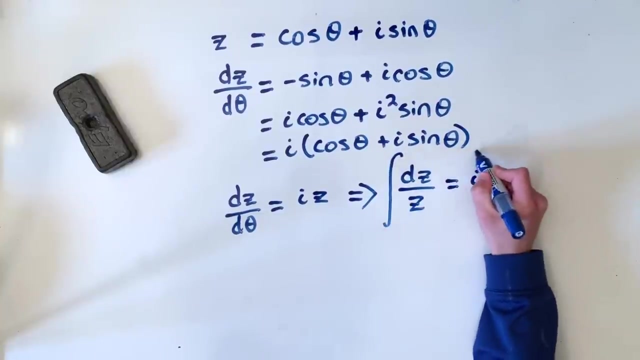 And now this is very easy, useful, because what we can do is we can rearrange that so that we have dz over z is equal to i d theta, and now with this we can integrate both sides like that, and the integral of one over z with respect to z will be the ln of z. 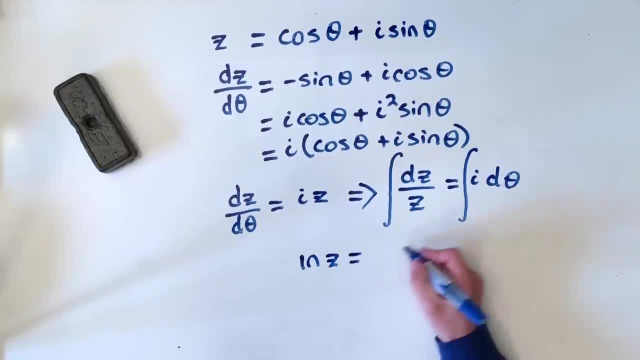 which will be equal to i as a constant times theta plus the constant c. now we do e to both sides, so we are left with: z is equal to e to the i theta plus c and we'll write c as e to the c, or just times that constant c.